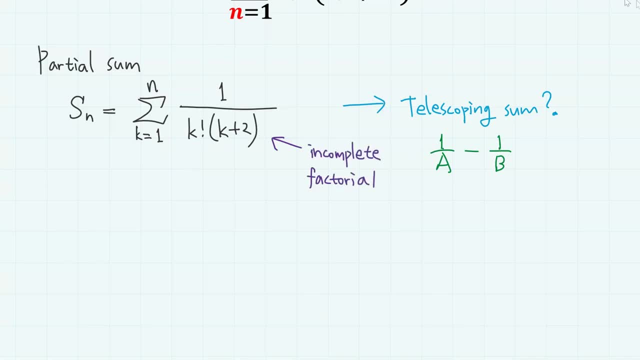 Is k factorial times k plus 2?, So it is some kind of incomplete factorial. Why? Well, if we only had additional k plus 1, this entire thing could become k plus 2 factorial. But we can forcibly make k plus 2 factorial anyway. We multiply k plus 1 in the denominator. 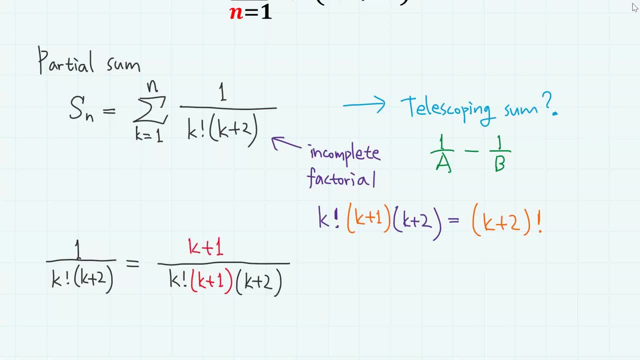 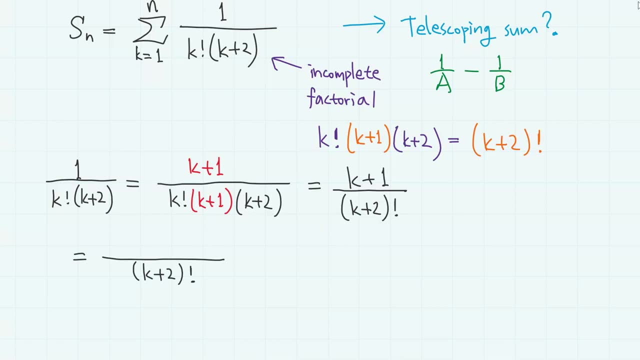 and we multiply k plus 1 at the numerator too, Then the denominator becomes k plus 2 factorial. Then we change the numerator Into k plus 2 minus 1.. Then we finally obtain a difference form, which is k plus 2 over k plus. 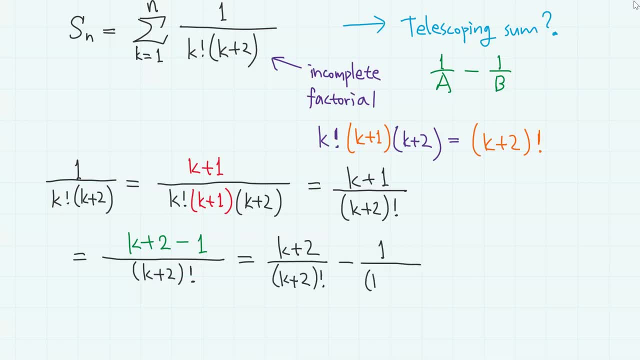 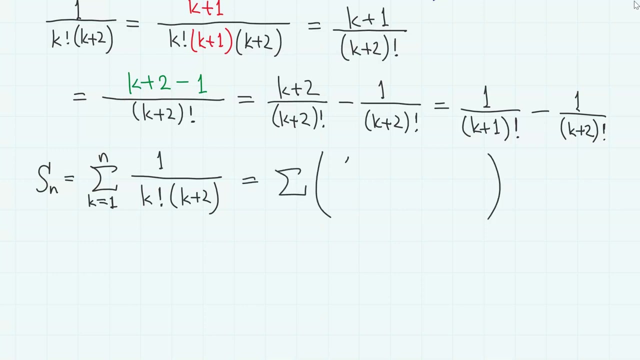 2 factorial minus 1 over k plus 2 factorial. And the first term is simply 1 over k plus 1 factorial. So we have 1 over k plus 1 factorial minus 1 over k plus 2 factorial. Therefore the partial sum Sn equals sigma 1 over k plus 1 factorial minus 1 over k plus 2. 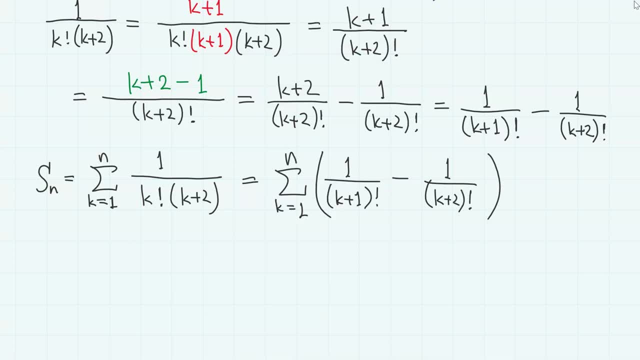 factorial from k equals 1 to n, So it is 1 over 2 factorial minus 1 over 3 factorial plus 1 over 3 factorial, minus 1 over 4 factorial plus 1 over 4 factorial, So it is 1 over 2 factorial minus 1 over. 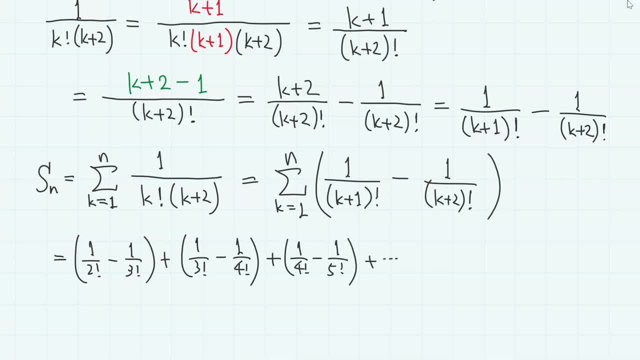 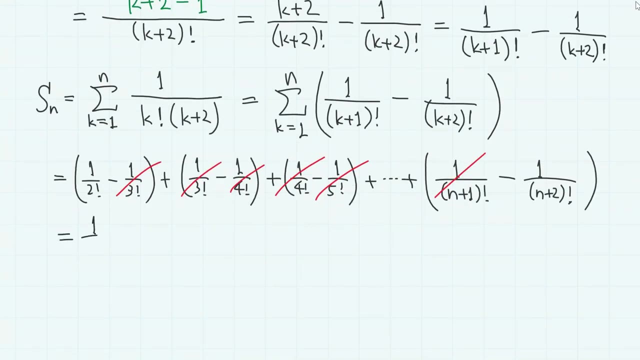 4 factorial minus 1 over 5 factorial and so on, And in the last part we have 1 over n plus 1 factorial minus 1 over n plus 2 factorial And, as you can see, the terms cancel out And we have 1. 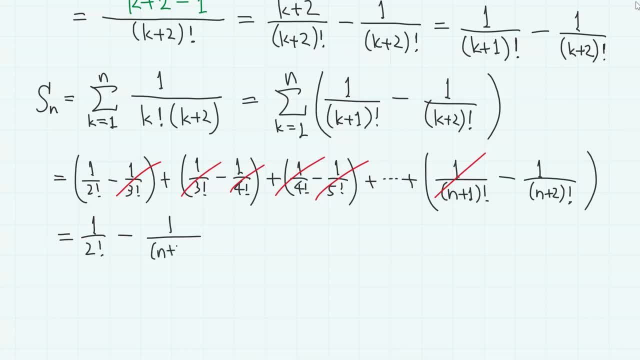 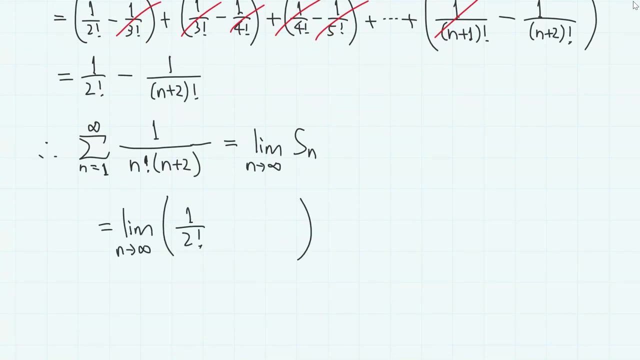 over 2 factorial minus 1 over n plus 2 factorial. Therefore the sum of this series is limit of the partial sum. Sn equals sigma 1 over k plus 1 factorial minus 1 over k plus 2 factorial. So limit of 1 over 2 factorial minus 1 over n plus 2 factorial, And this part goes to 0. So we